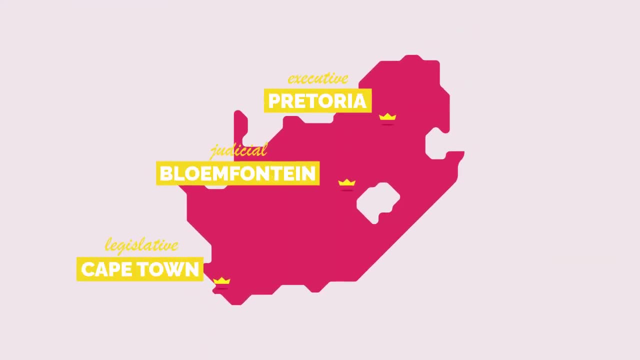 as shown, The country has three capital cities. The executive capital is called Pretoria. However, the largest city is Johannesburg, with almost nine million people. This city also acts as the main hub for the country, due to its airport being the busiest in all of Africa. 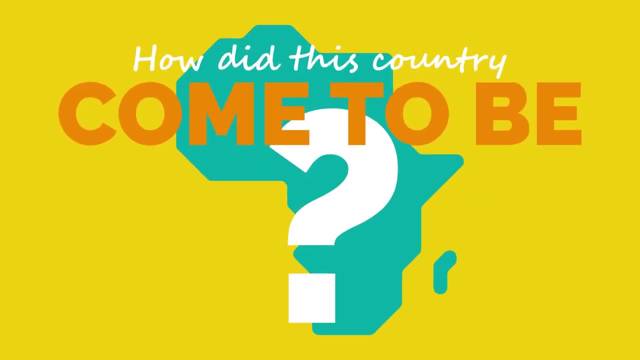 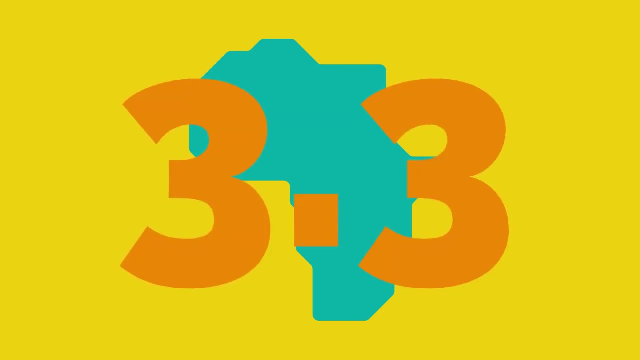 But first things first. how did this country come to be? Well, the origins of South Africans really don't have a starting point, since humans have been roaming Africa for some 3.3 million years. But it is known that the last of these humans, called the Bantu people, were present in the 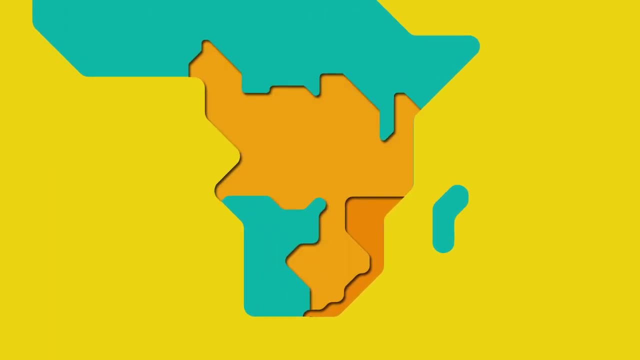 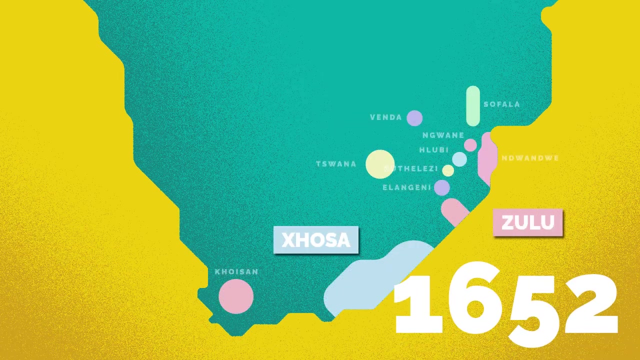 eastern lowlands. They are thought to have come from central Africa, displacing and assimilating local tribes as they came down. Two main clans descending from this Bantu people are known to have been present when the first European settlers came, But they didn't have. 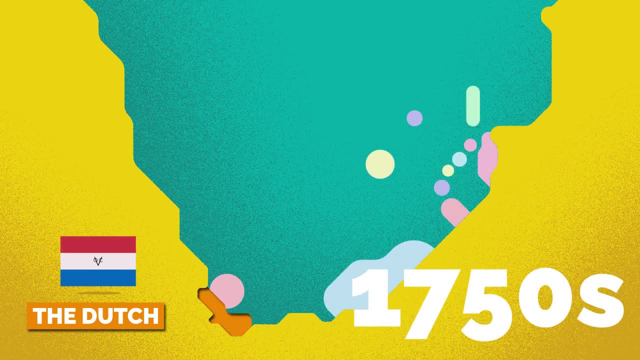 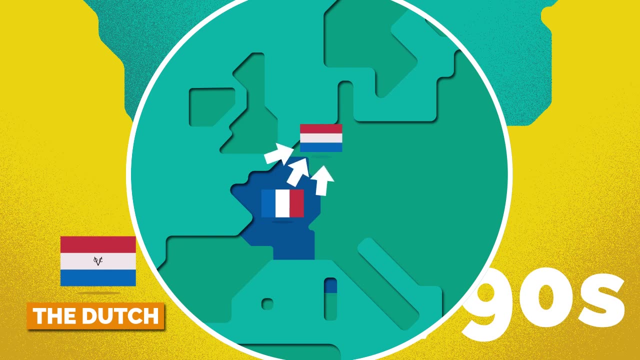 contact until a century later, when the European expansion reached their lands. Meanwhile, Europe was having its own share of expansion issues. France invaded the low countries, which meant that the Dutch colonies were in danger as well. So the British took over to prevent France from. 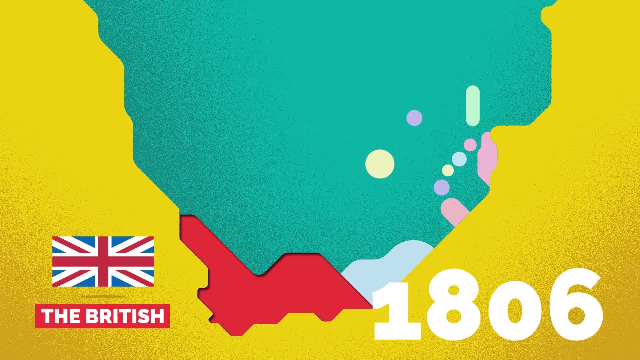 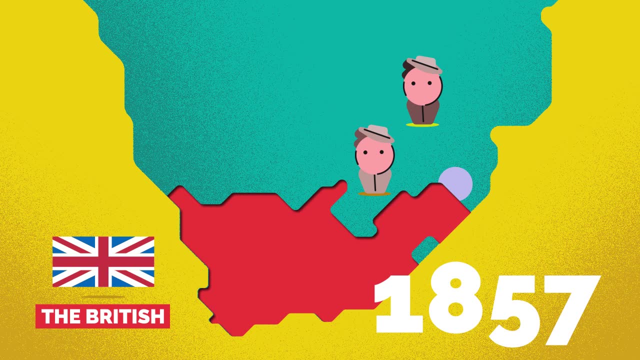 having possessions down there. This, however, would destabilize the region, because many Dutch descendants that had been living there since the 1600s fled British rule. due to discontent, They formed their own republics further north, but still eventually fell into British hands. 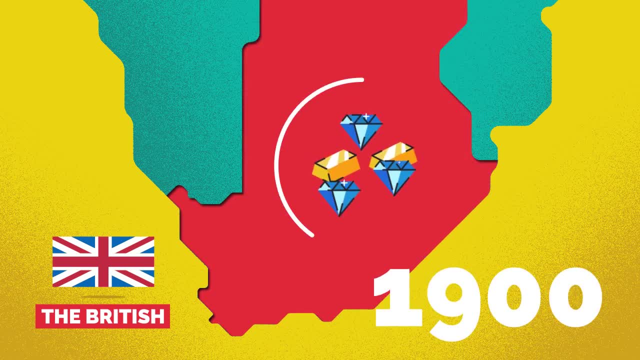 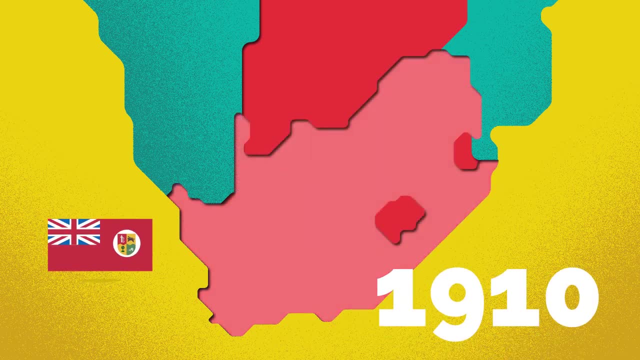 This led to more indigenous tribes. thanks to the discovery of diamonds and gold in the region, Flashes inside the territories were common, so the whole country was given a degree of autonomy in 1910 to ease the tensions inside. It became a self-governing dominion of the British Empire. 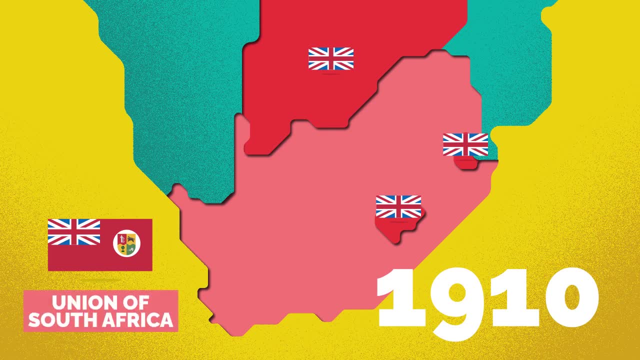 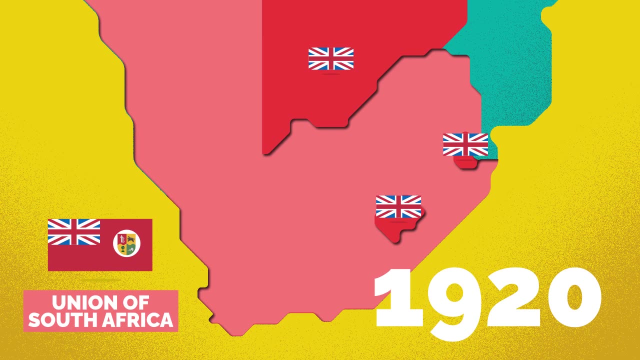 much like Canada or Australia, called the Union of South Africa, And the South Africans were also given a big piece of land to administer as a result of Germany losing World War I. But it wasn't enough. They sought independence, and it was achieved in 1931,. 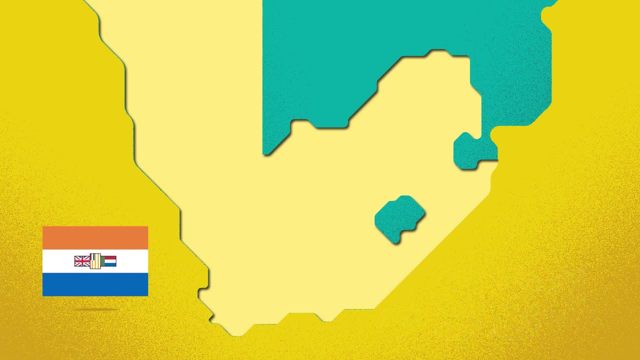 although not for all people, because racial segregation was present in South Africa. In fact, this segregation was codified at an institutional and legal level. in the 1950s, This was known as the Apartheid, where the white minority enjoyed a high standard of living. 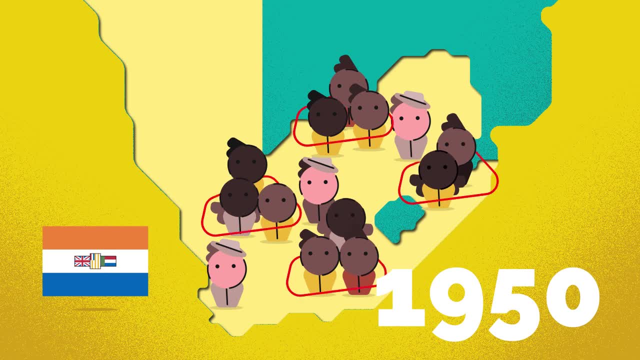 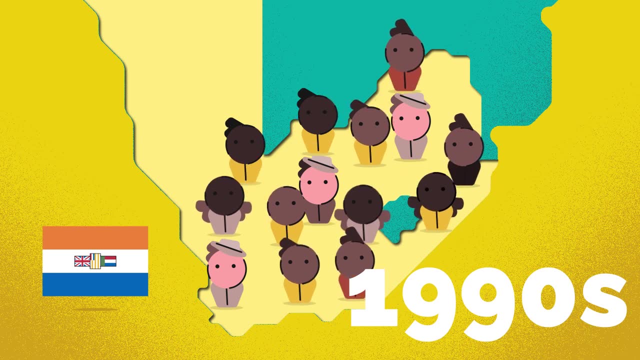 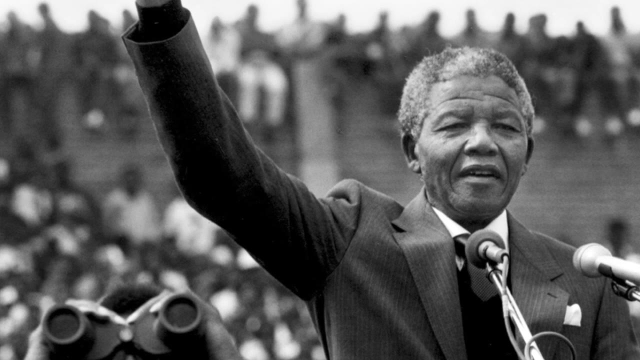 and the black majority remained disadvantaged by almost every standard. It wasn't until the 1990s that the fullest expression of an independent state came true, when people from all backgrounds voted and decided their own future. Nelson Mandela, the first universally elected president of the Republic of South Africa, would be the figure that would 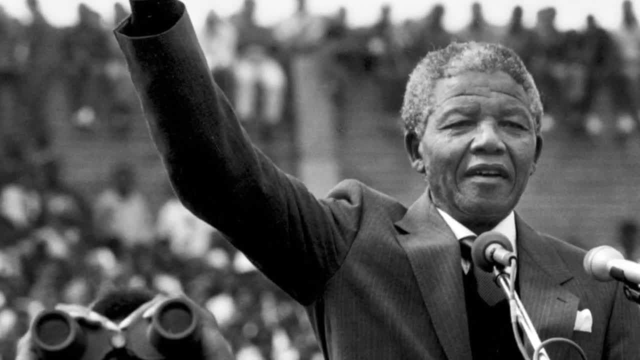 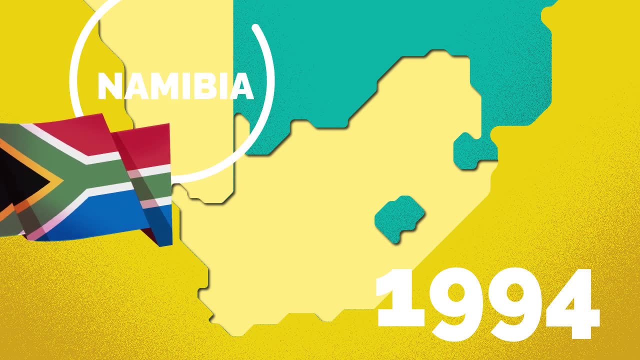 achieve the historically rare feat of uniting a fiercely divided country by showing the world how to respond to injustice and tragedy. By the way, by this time, that huge chunk of land in the West was already given independence, So the borders have remained the same since the 90s. 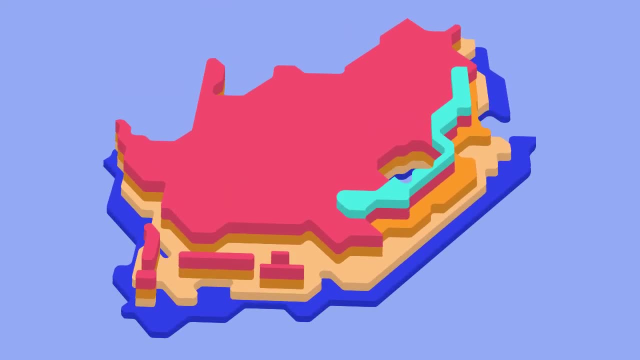 but what does it look like on the inside? The interior of South Africa consists of a vast, in most places almost flat, plateau, with the highest peak located on the border with Lesotho at 3,450 meters above sea level. The edge of the plateau is also characterized by steep slopes. 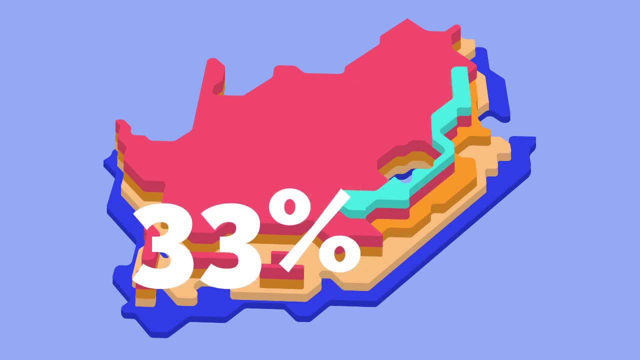 filled with grassland over these areas. Over 33% of the land area is filled with what we call savanna, which is characterized by a grassy ground layer with some woody plants on top. The western side of the country has two zones with semi-desert characteristics. 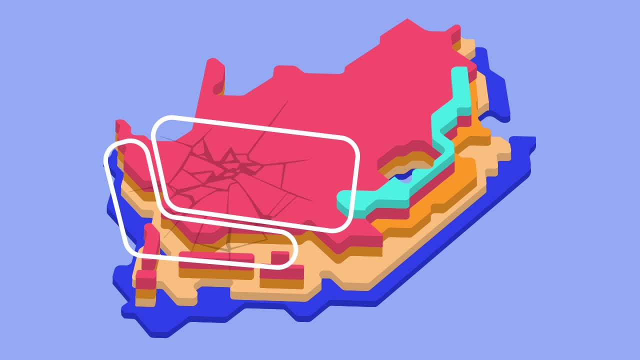 such as extreme aridity. The difference between the two is that one receives the little rain that falls as cyclonic rainfall in winter, which has less erosive power than the infrequent but violent summer thunderstorms of the other. Lastly, we find this belt of natural shrubland vegetation. that clothes the mountains and lowlands of the Cape. Enormous diversity of species of flora are present, making it a unique environment that is not found anywhere else in the world. To add to these, we also find national protected areas and parks filled with thousands of species. 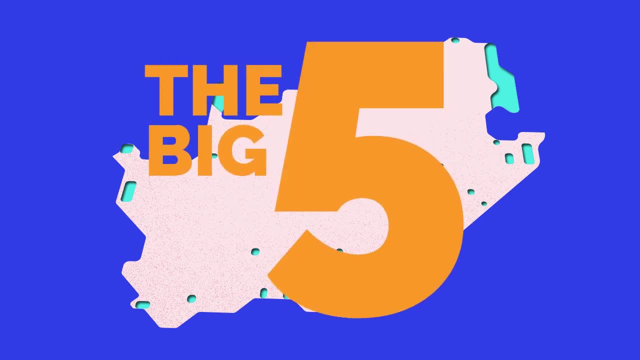 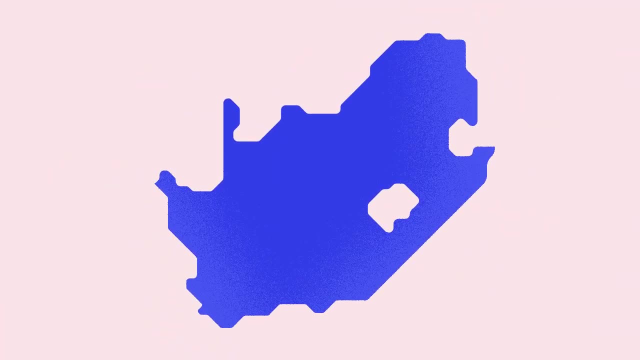 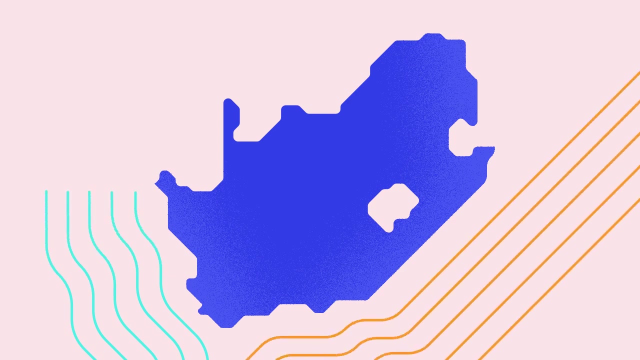 of wildlife, including the Big Five, which includes the African elephant, the Cape buffalo, the lion, the black rhino and the leopard. Climate-wise, South Africa is a relatively dry country. The currents of both the cold Atlantic Ocean and the warm Indian Ocean influence the 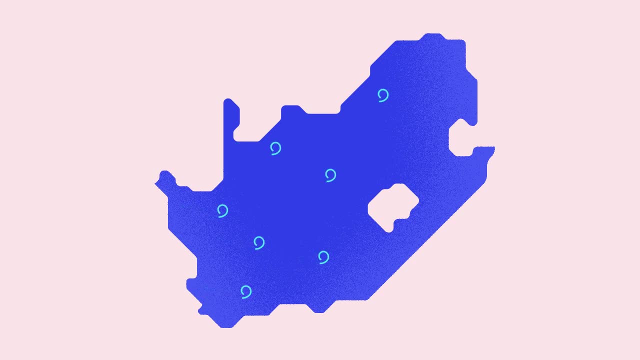 rainy season. In the western parts, the cold air cannot hold a lot of moisture, so there is little precipitation. The opposite happens in the east, where the warm air holds more moisture and more rain falls throughout the year, Regardless of where it falls. if we were to gather all rainwater in South Africa? 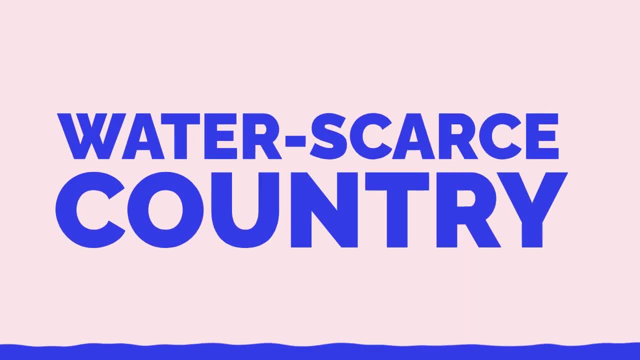 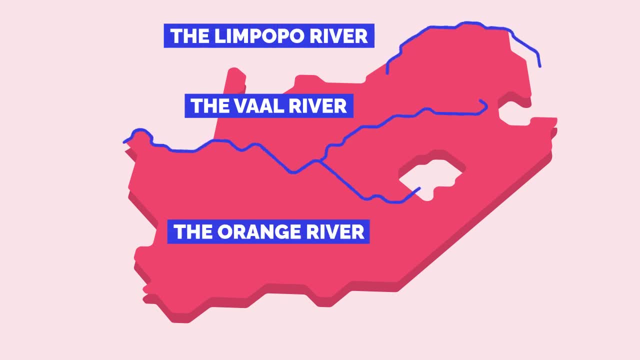 it would still amount to very little, Which is why it is recognized as a water-scarce country. Not even the main rivers — the Val River, the Orange River and the Limpopo River — can help with the lack of fresh water. 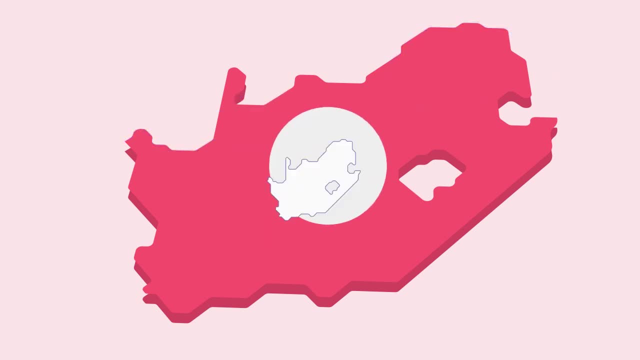 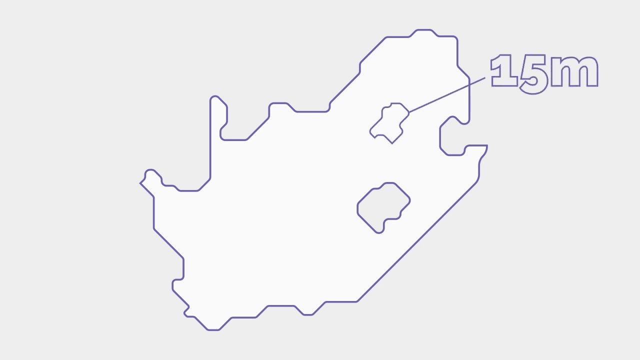 Increasing population makes it even more difficult, especially in the big cities such as Johannesburg, which is, as previously noted, the biggest. It is part of the province of Gauteng, home to 15 million people. Together with these eight other provinces, South Africa is home to 57 million people. 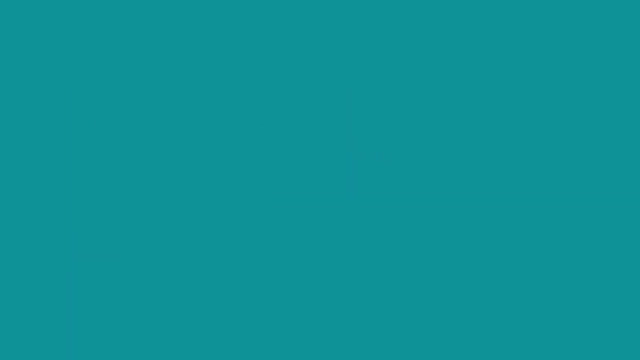 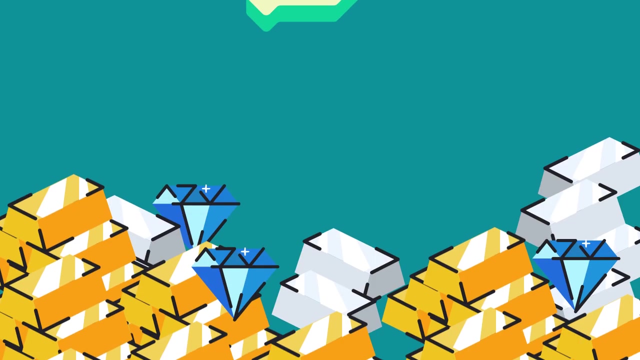 When it comes to the economy and how the people of South Africa keep moving the country forward. well, you could sum it up with one word — minerals. South Africa is richly endowed with mineral resources, most of them found in the central region. They represent 54% of all exported goods, including precious materials such as diamonds. 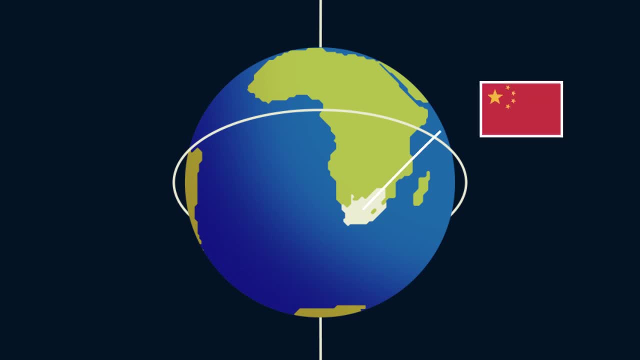 gold and platinum. The main export destinations are China, representing 16% of the total share, the UK with 8% and the US with 7%. China is also the main origin of imports, with 18% of the trade. 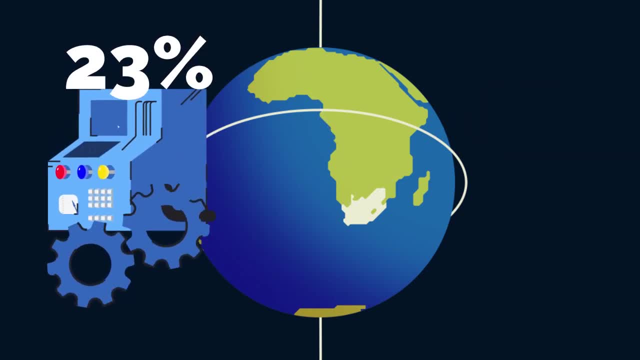 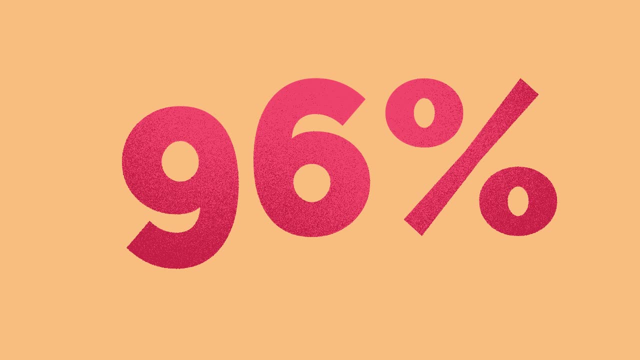 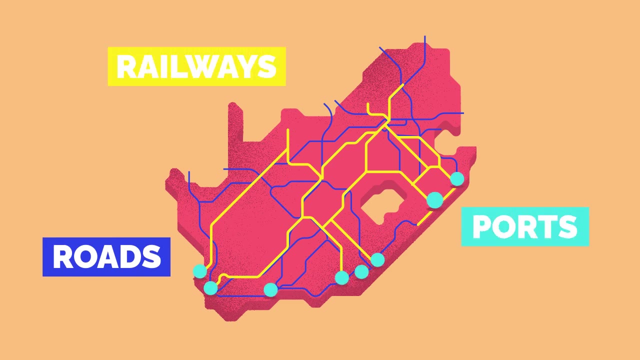 Germany and the US. Goods from these countries include machinery, petroleum and transportation-related items. 96% of the country's trade is conveyed by sea, which is why a well-connected network of roads and railways must support the important ports across the coast. After all, the shipping route just south of the nation is still a major 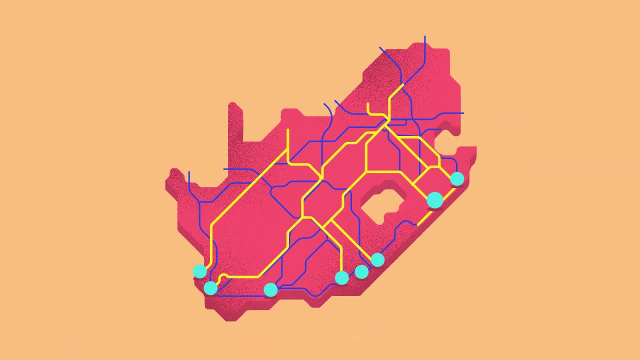 global trade route When it comes to transportation of people. well, you could go from the capital city of Pretoria to Cape Town by car, but it would take you almost 15 hours. You could also consider air travel through one of the many airports the country has. 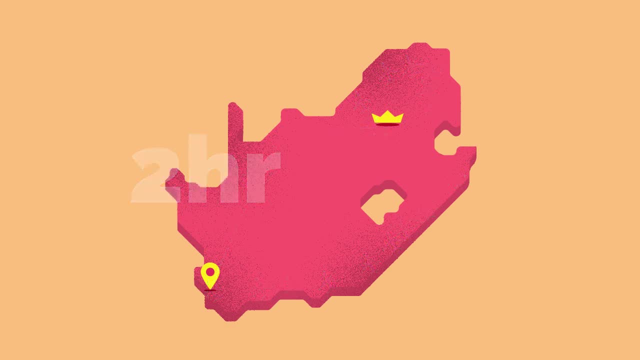 and reduce the time to two hours, But then you would miss all the magnificent scenery South Africa has to offer. The best of the alternatives if you don't want to miss any piece of landscape is definitely taking trains. It does take about 26 hours, but it is more than. 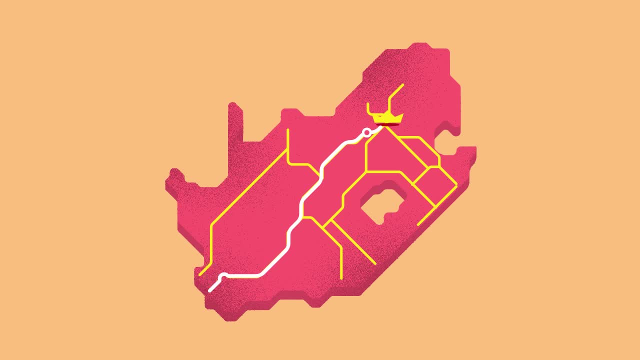 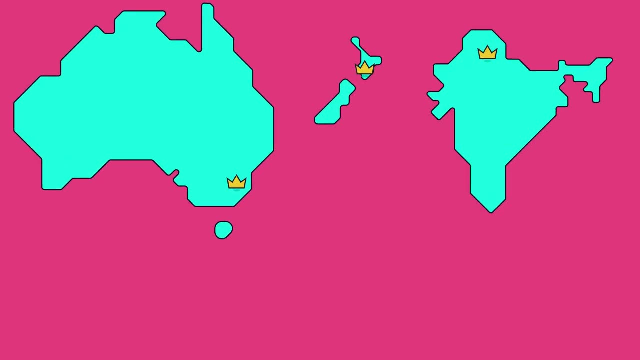 just a means of transportation. It's an experience. We've reached the end of the video, but we can't leave without addressing the friendships and rivalries this country has. South Africa's biggest rivals are probably more related to sports than anything else: Australia, New Zealand. 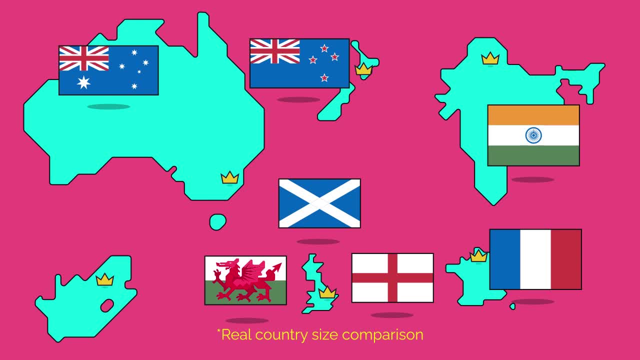 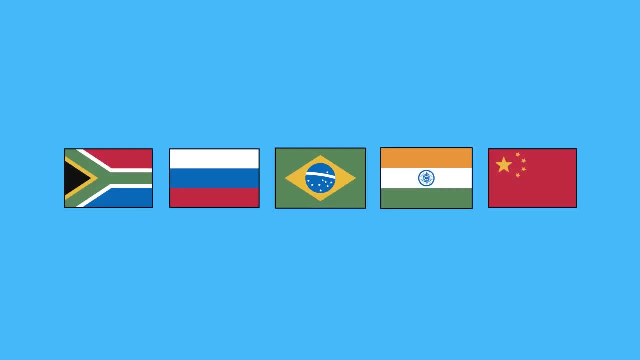 France, India and Great Britain would be the title bearers, as they are South Africa's largest competitors in rugby and cricket And, when it comes to friends, their main allies are definitely the BRICS countries, whose cooperation was driven by their shared identity as emerging economies.